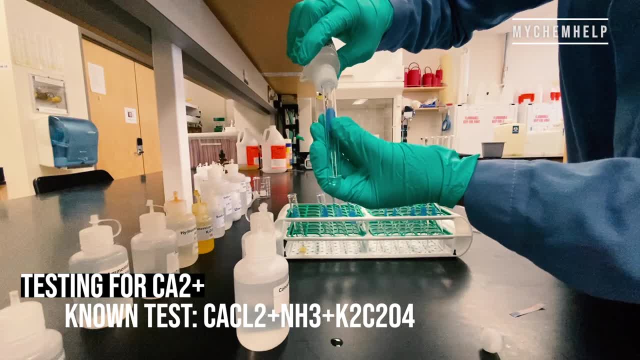 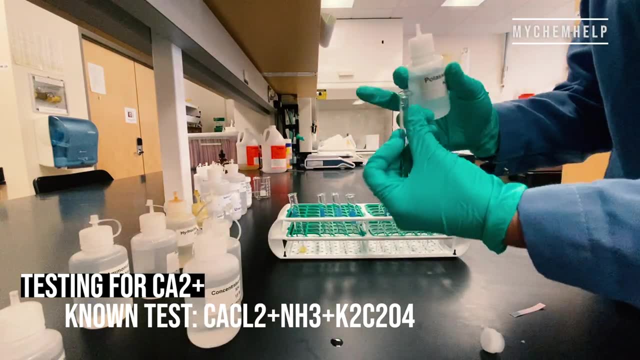 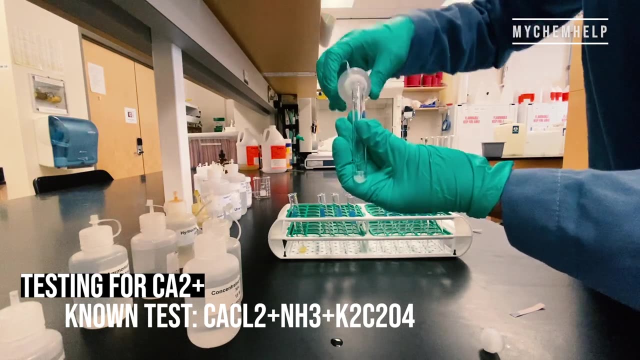 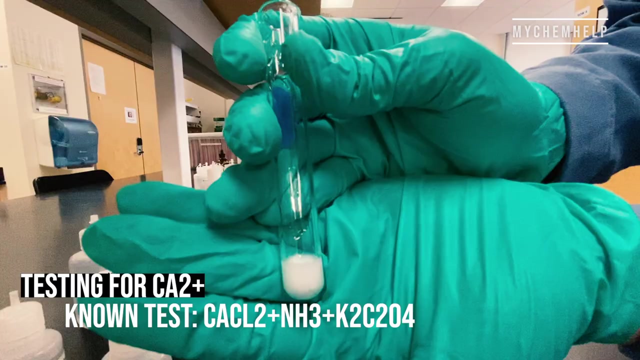 of that solution onto the paper. It's blue, so it indicates that it is basic. And lastly, I'm going to add some potassium oxalate to the solution, And that white precipitate there signifies a positive test on this one. So now we're testing the unknown. 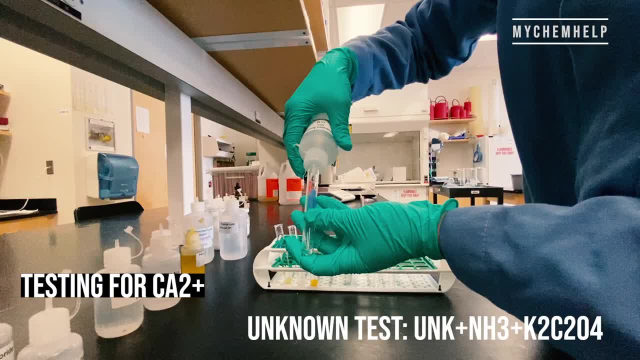 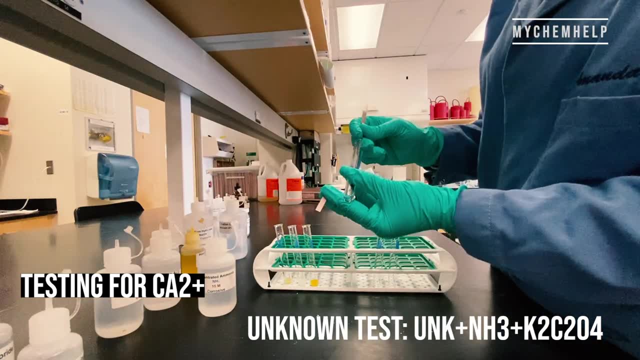 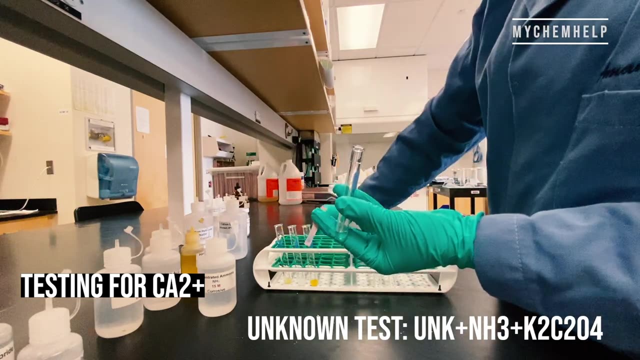 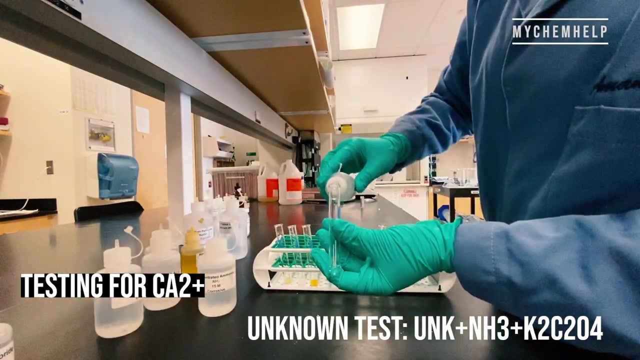 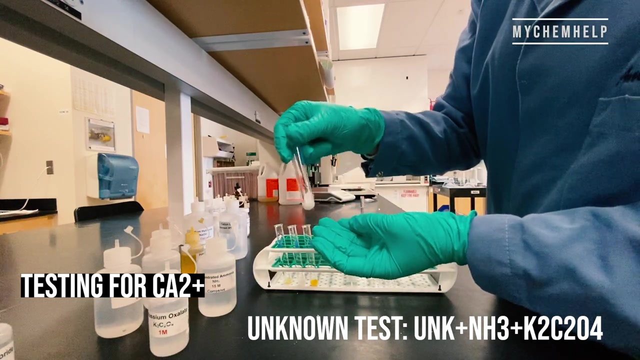 It's our unknown solution, followed by ammonia, And again I'm going to test to make sure that it's basic Yep. And here's our unknown solution And a few drops of potassium oxalate. And, like I said in the beginning, I'll let you guys come to your own conclusions about these unknowns. 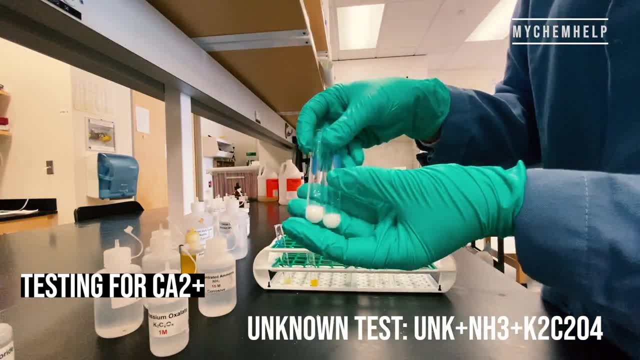 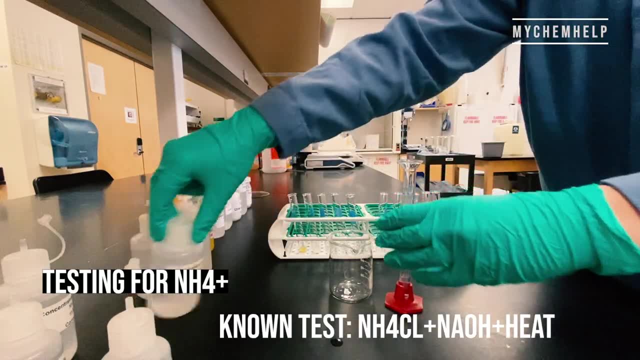 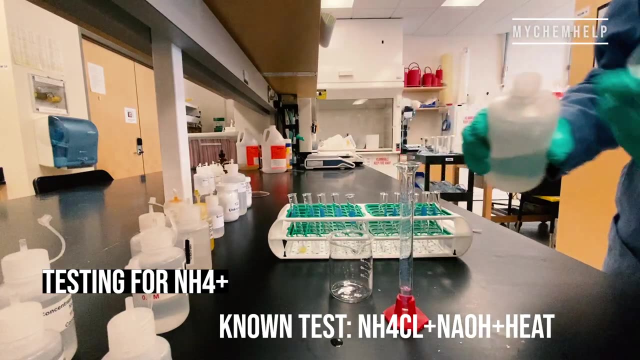 So maybe if you want to follow along and write down observations, then maybe you could find out what the unknown is or maybe hypothesize about what you think it is. So next we're going to test for an ammonium ion. That's two milliliters of ammonium chloride followed by 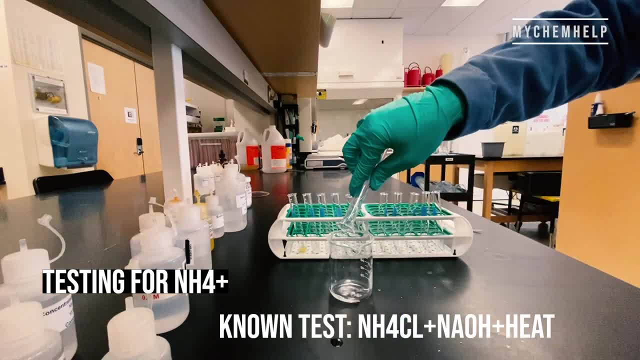 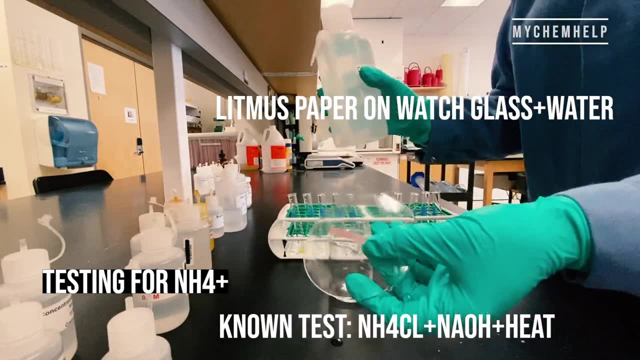 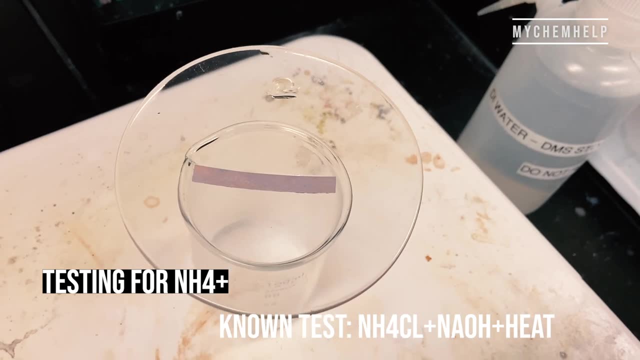 two milliliters of sodium hydroxide and that's going right into the beaker as well. And then I've got litmus paper on a watch glass. I'm just going to adhere it to the surface with a bit of water and stick it on top of that beaker. We're gently heating it to see if the vapors turn the. 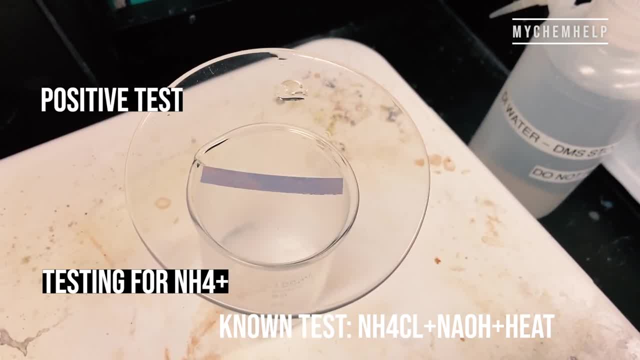 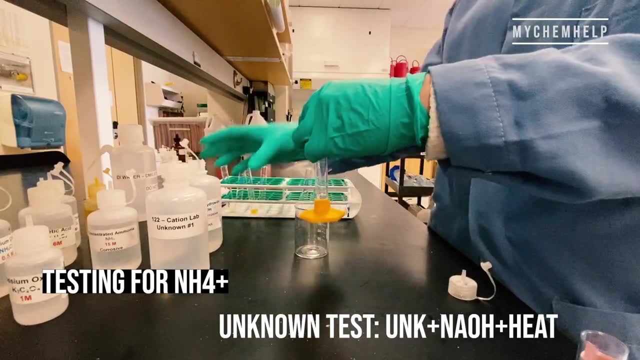 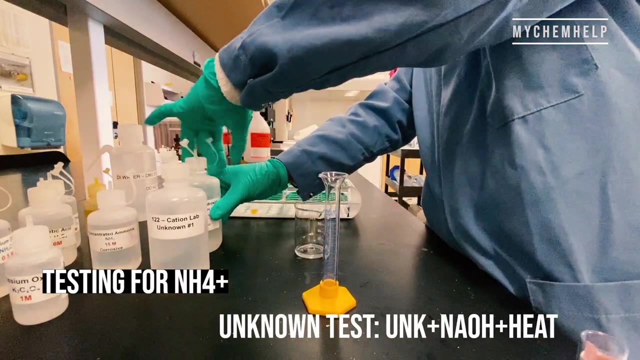 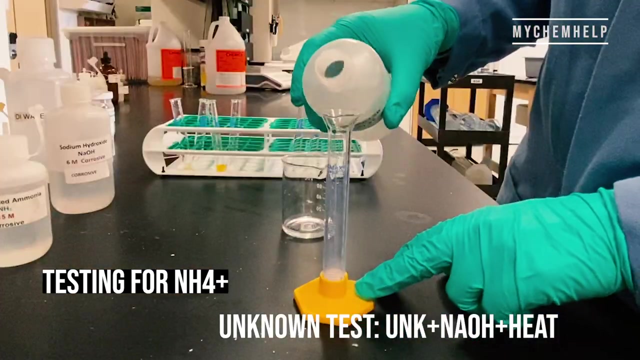 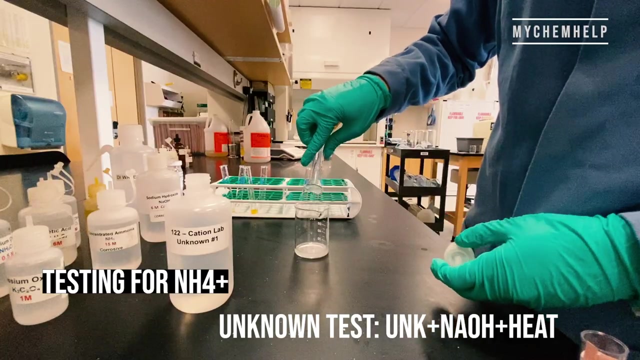 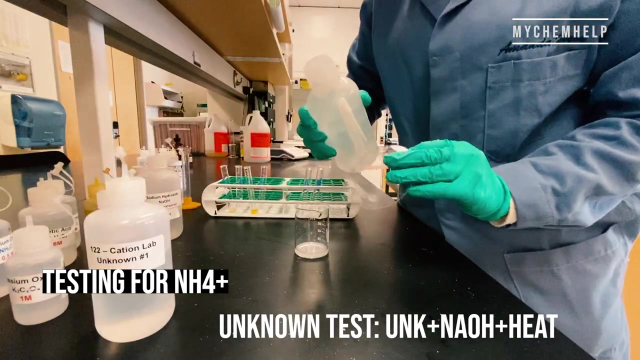 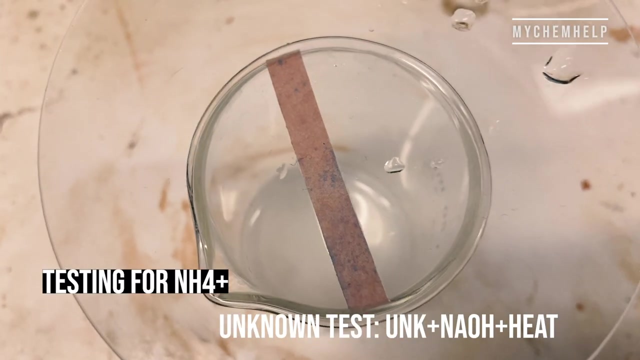 litmus paper, blue, And we've got a positive test there. So now we're doing the same process with our unknown. Oh, wasn't expecting that to happen. Wash glass, litmus paper, All right. so now let's put that on a hot plate and see what happens. 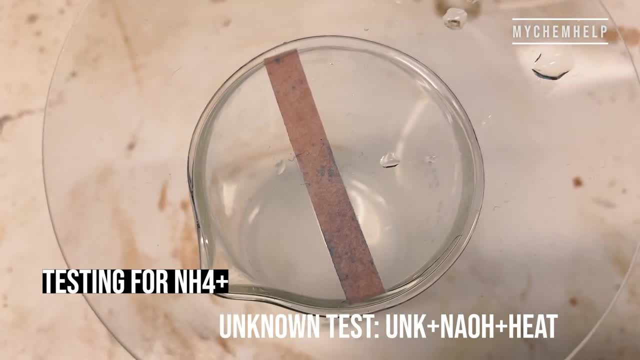 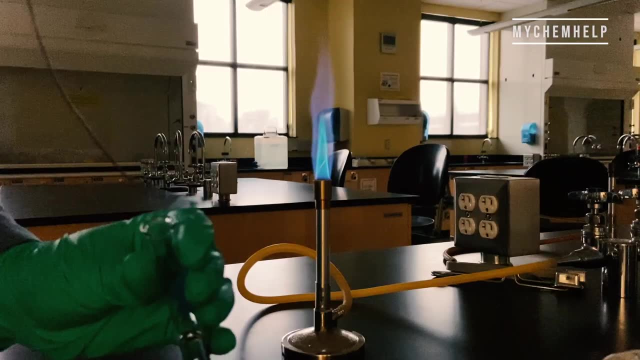 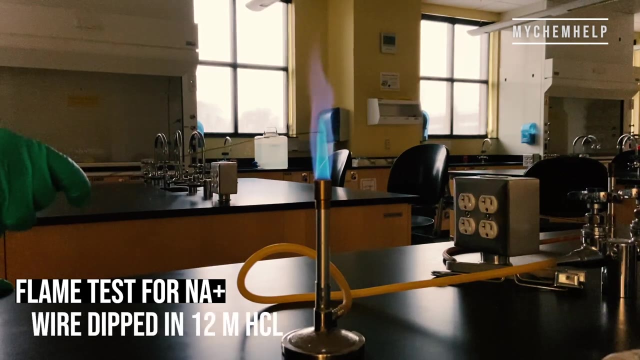 I'm not so sure about this one. What do you guys think is happening? And for our last test, we're going to put it on a hot plate and see what happens. We are doing a flame test. So this is for sodium ions. So first I'm cleaning the nichrome wire. 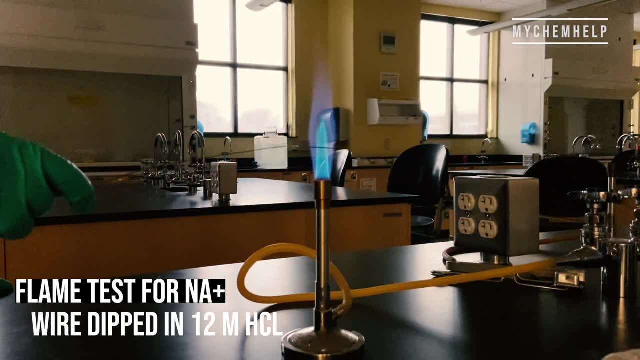 with 12 molar hydrochloric acid. It's a really cool flame And I'm going to repeat that until the flame is colorless, or basically just back to that blue color. All right, here's the wire. I'm going to put it on a hot plate and see what happens. 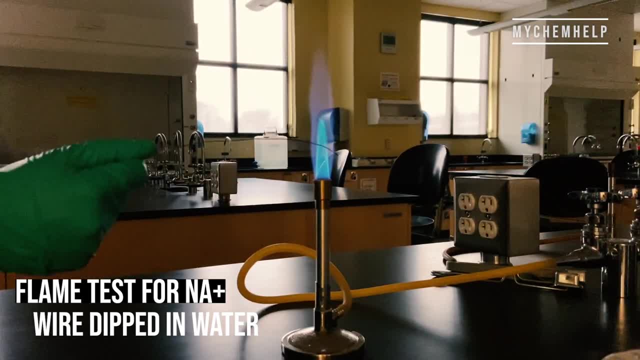 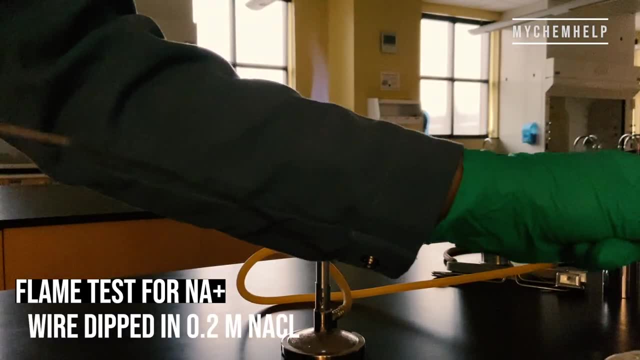 All right, here's the wire. I'm going to put it on a hot plate and see what happens. All right, here's the wire, dipped in water. Not much is happening there, And this is our 0.2 molar sodium chloride solution. 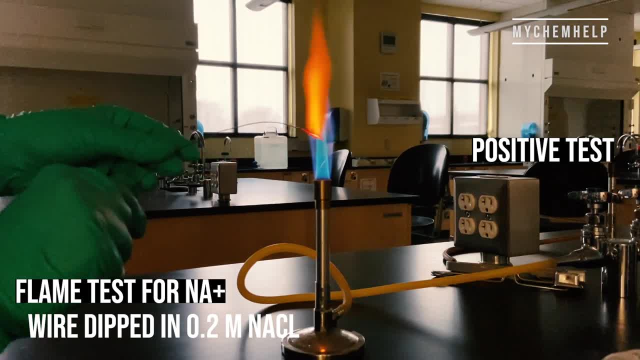 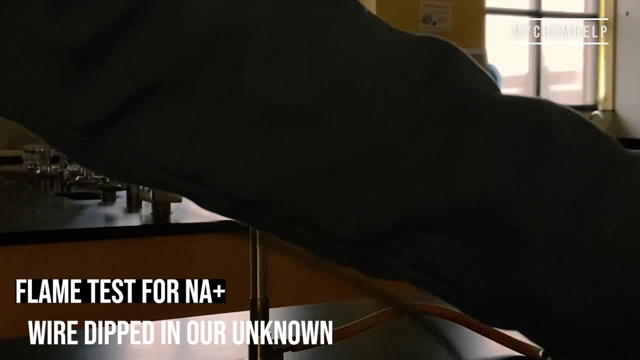 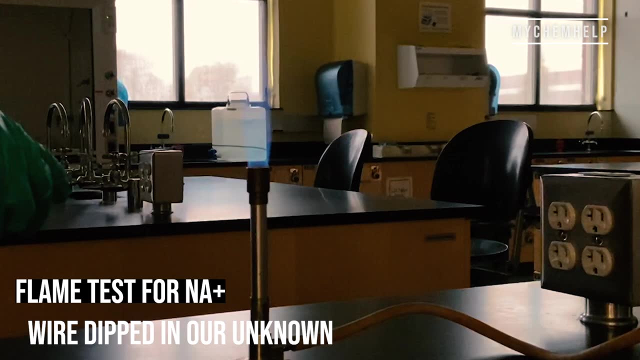 And this is a positive test here. You see that really bright yellow flame in the middle. That's exactly what we're looking for, All right, so now it's time to test the unknown, And I can't really see much happening. but I don't know. I'll leave that up to you guys. 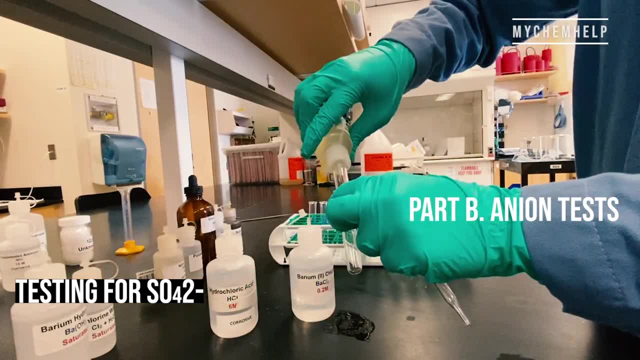 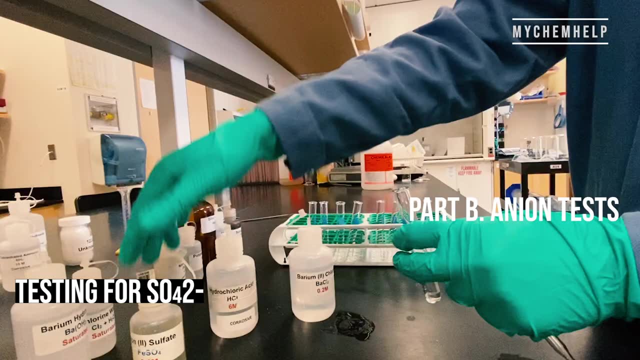 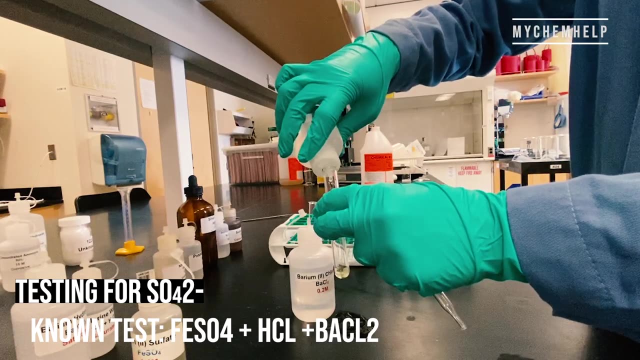 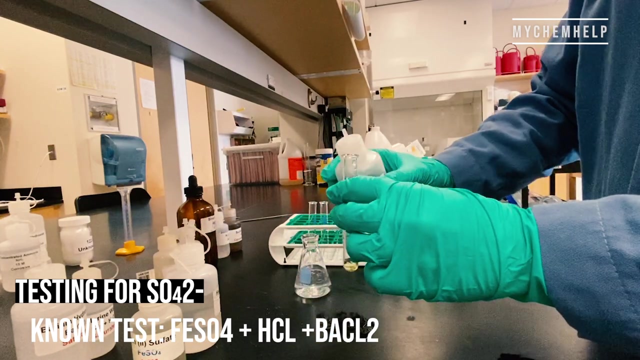 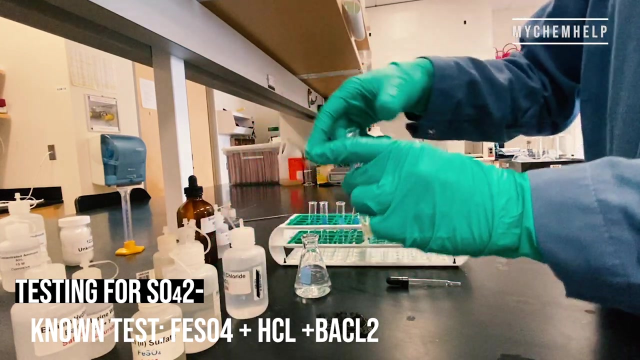 What do you think? Back into the lab for part B, We have the anion test. So here we're looking for sulfate ions And our known test is going to be iron sulfate plus barium chloride, And that white precipitate tells us that that is a positive test. 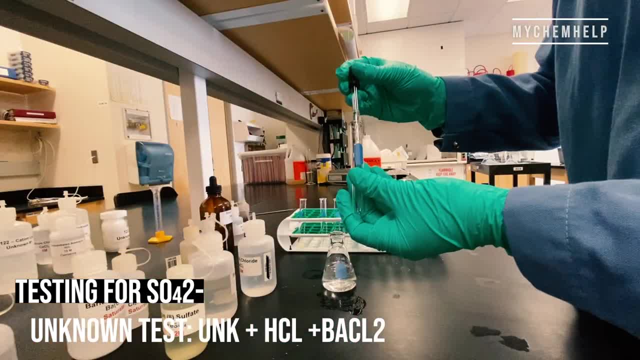 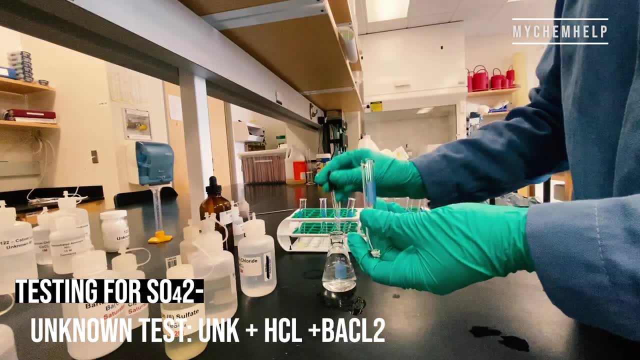 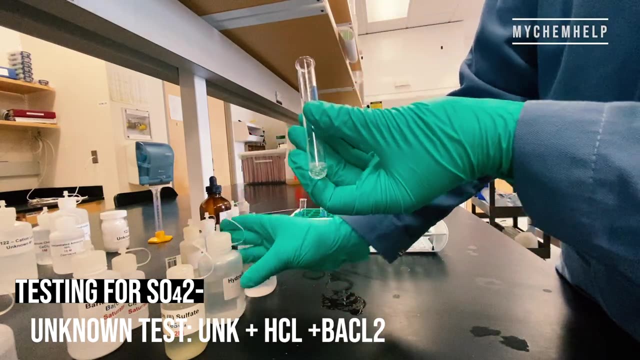 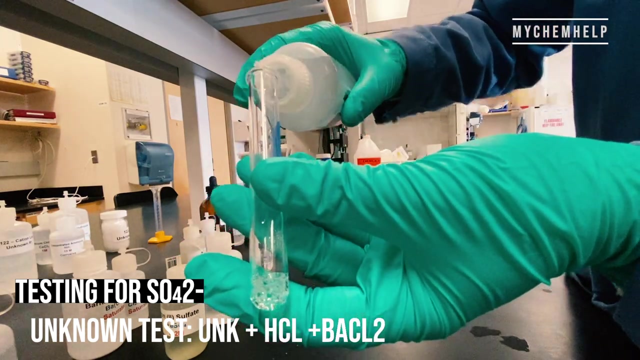 So now let's check out the unknown. So I've got my unknown solution in that flask there, Just dropping a bit into the test tube, Adding some more Adding some hydrochloric acid And it looks like some bubbles formed. There's that barium chloride. 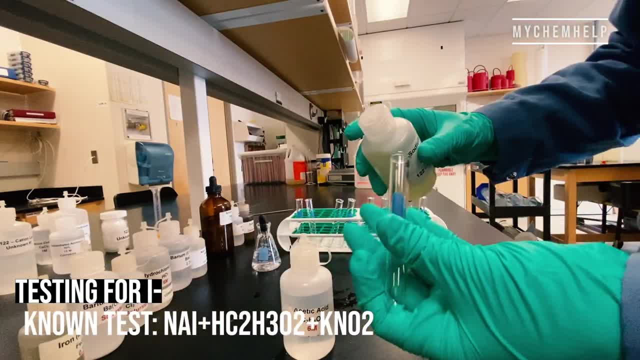 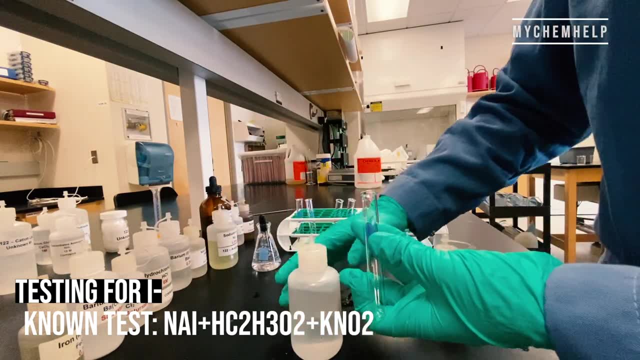 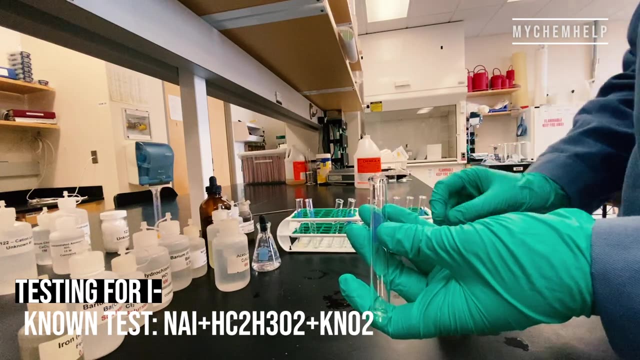 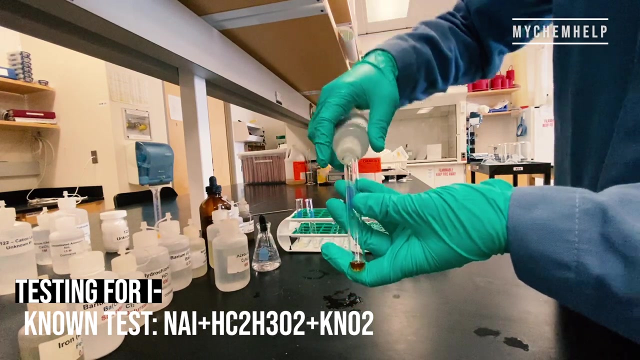 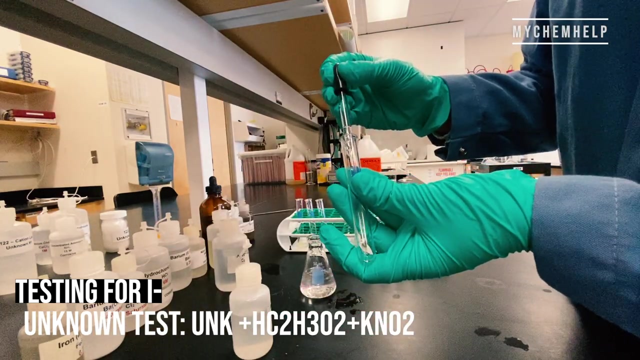 All right on to iodine. The known test is sodium iodide. That's what I just put in there with acetic acid Plus potassium nitrate, And the brown color indicates a positive test. Now let's test our unknown for iodine. 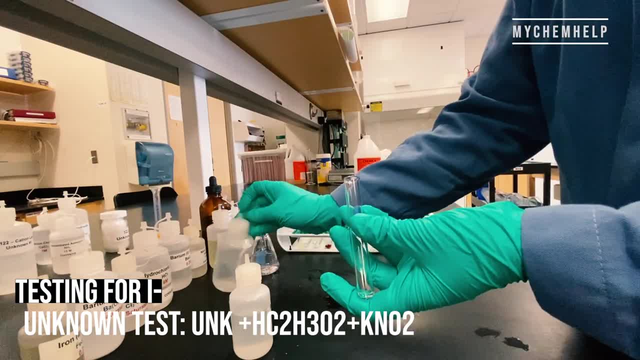 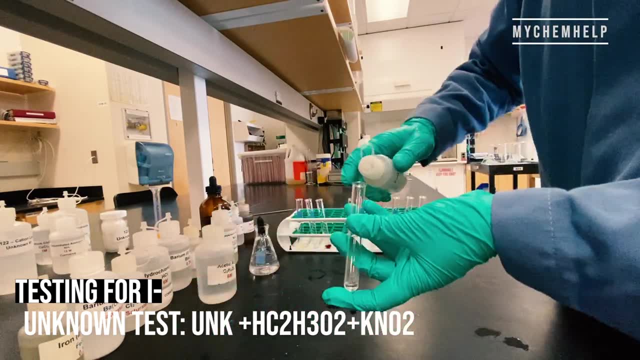 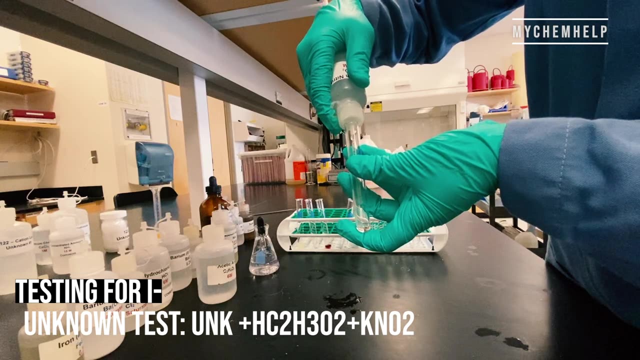 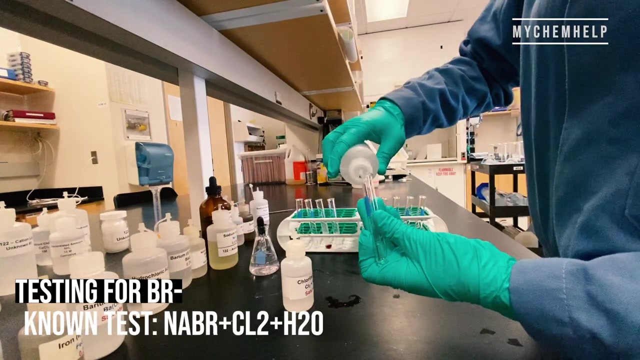 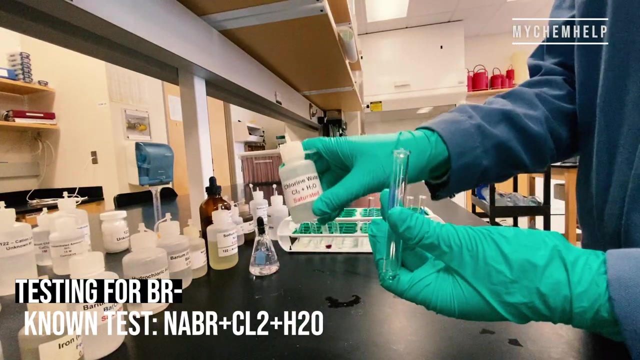 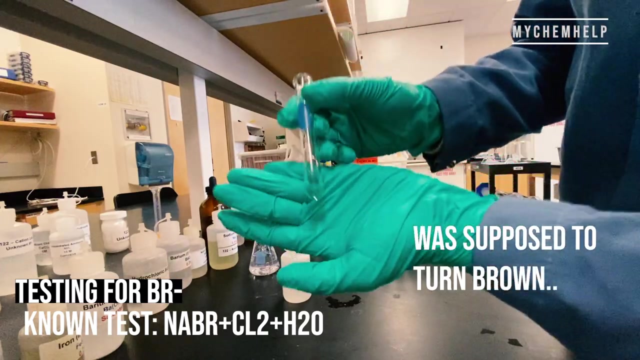 Let's test it And the brown color indicates a positive test. all right, now we're on to bromine. that's br minus and i am now we're looking for. into the test tube. i added sodium bromide plus chlorine water and that was supposed to turn brown. i'm not really sure what happened there. 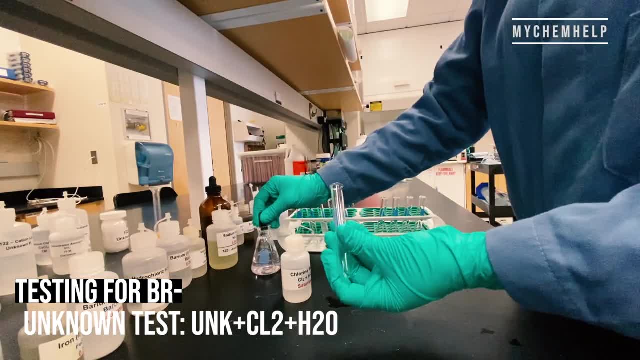 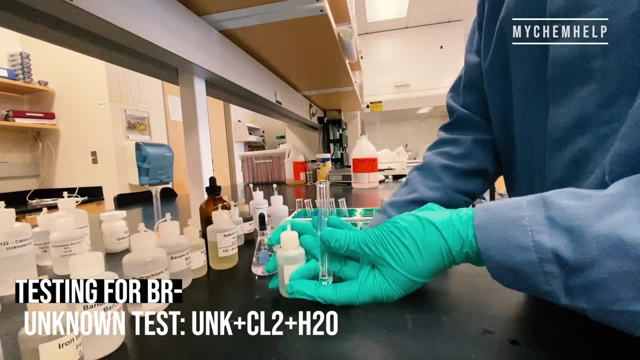 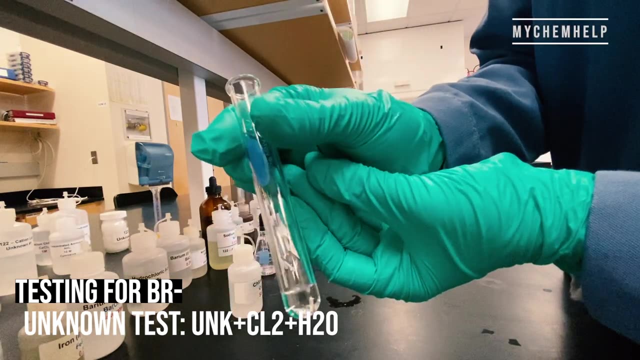 and even though i didn't see the reaction i was hoping for for the known, i'm still going to test my unknown and just to see what happens. and during qualitative analysis, stuff happens and stuff doesn't. um, it should be noted in your lab notebook that there was no visible reaction, as opposed to no reaction, because we can't actually 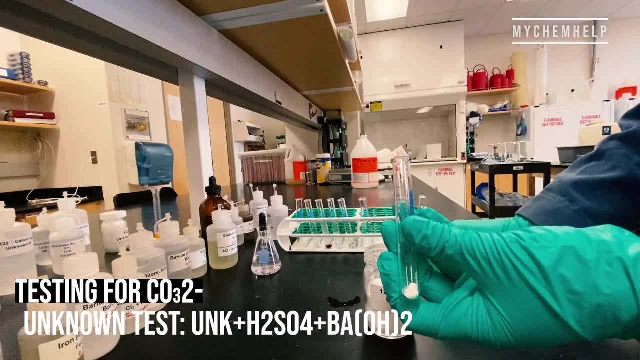 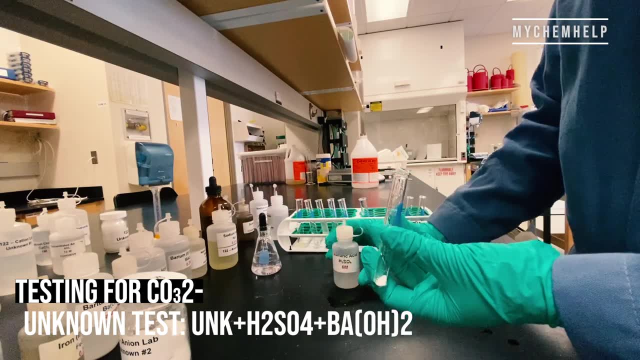 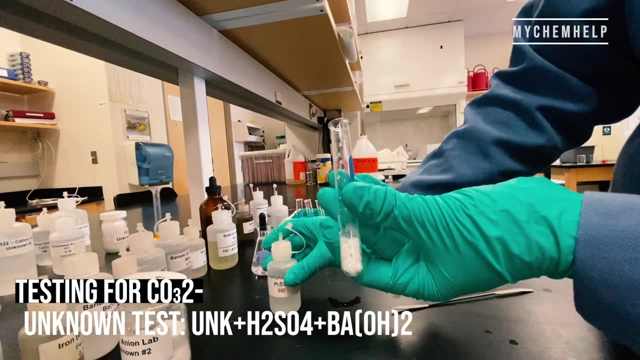 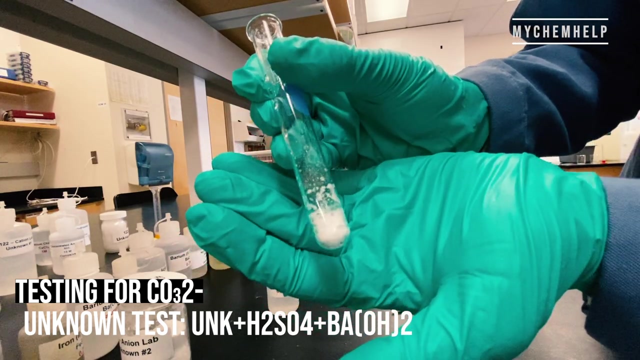 tell if there was a reaction happening or not. all right, so the next test is for the carbonate ion and i just went ahead and did the unknown test because i was really pressed for time. anyway, there's the unknown solid with sulfuric acid and in the lab notebook it said we should see gaseous evolution with the addition of sulfuric. 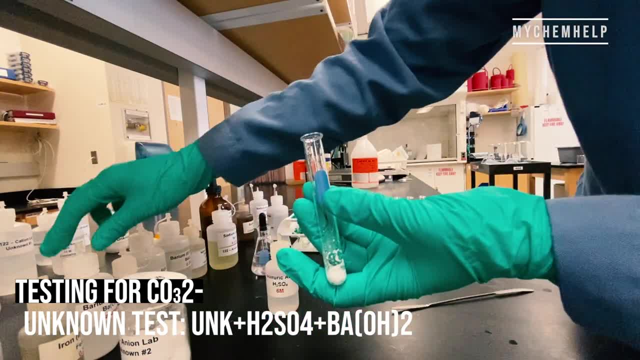 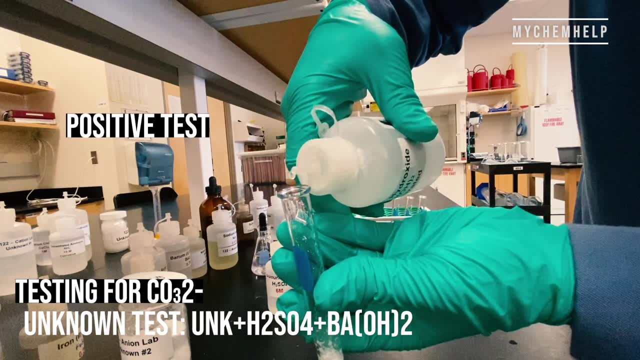 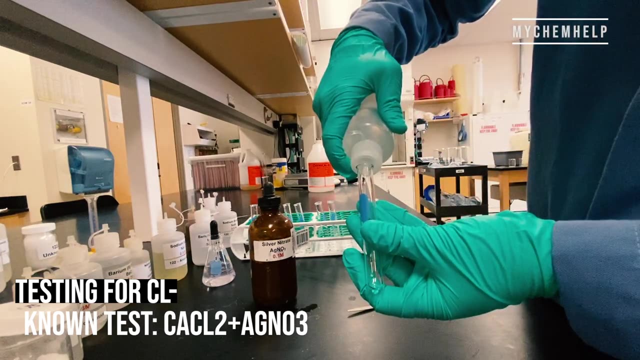 acid. and i'm taking a drop of barium hydroxide over the top of the test tube to see if it turns milky, and we've got a positive test there. so i'm next testing for chlorine ion. let's see l minus. and i've got calcium chloride going right into the tube with some silver nitrate.